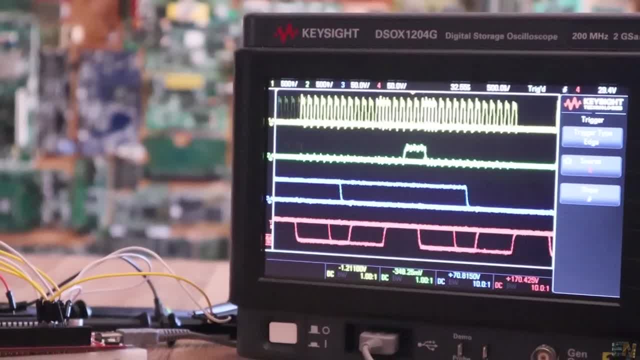 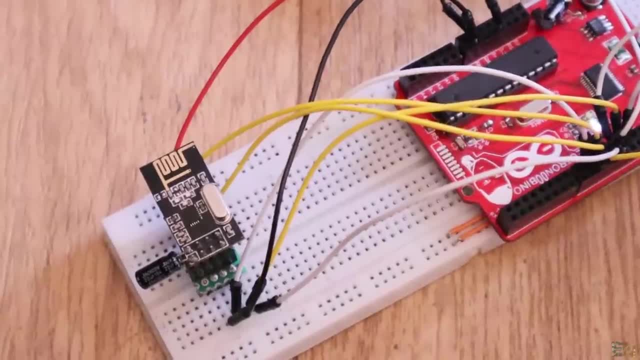 Wired communication, I2C and SPI. I will tell you the main characteristics of each one of these, show you how they work and why use one and not the other, and also show you a small example using the Arduino. We should also see the signals on the oscilloscope in order to get a better view. 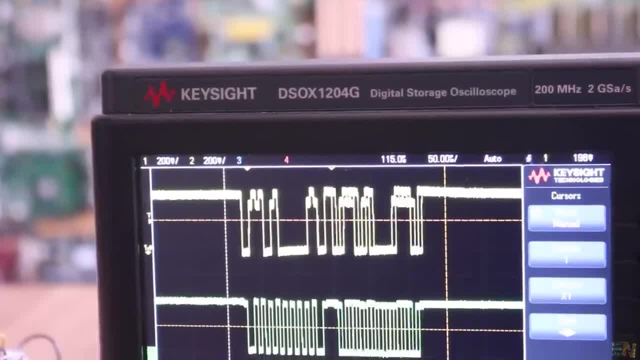 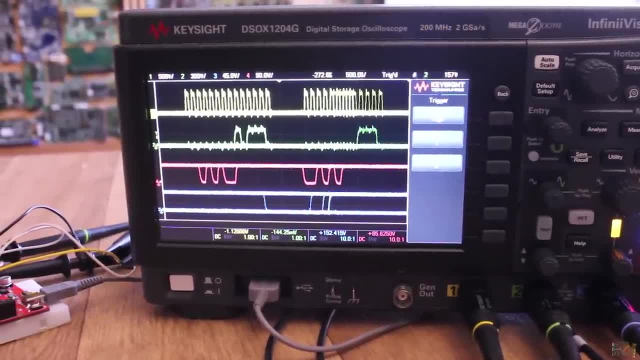 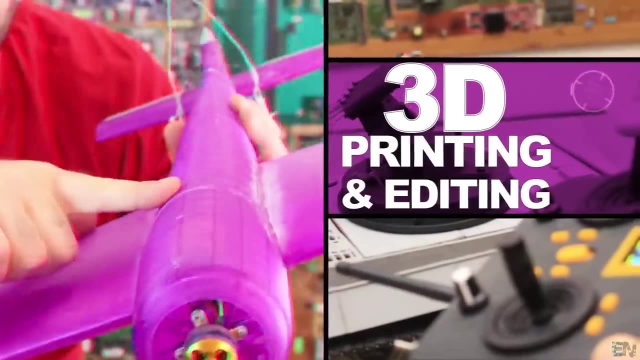 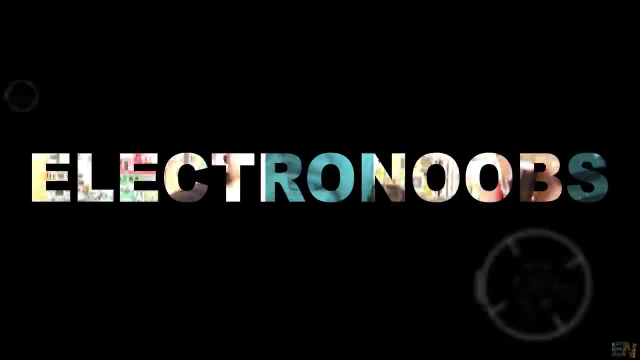 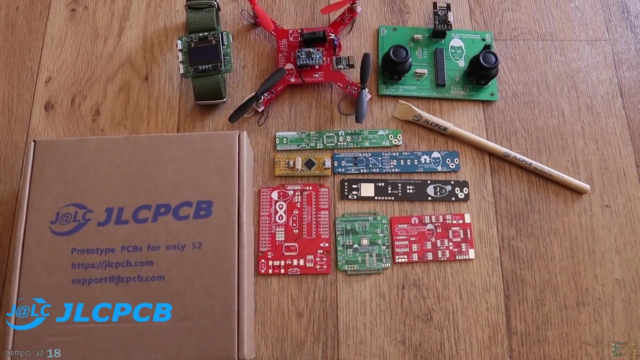 and by that understand more. So let's see how the Wired I2C and SPI work, but before make sure you subscribe and activate the notification bell. Thanks to all my patrons for the support. The sponsor of this video is JLCPCB. Thanks to all users' feedback. 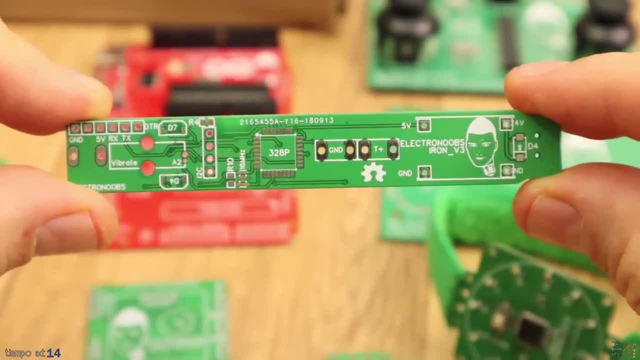 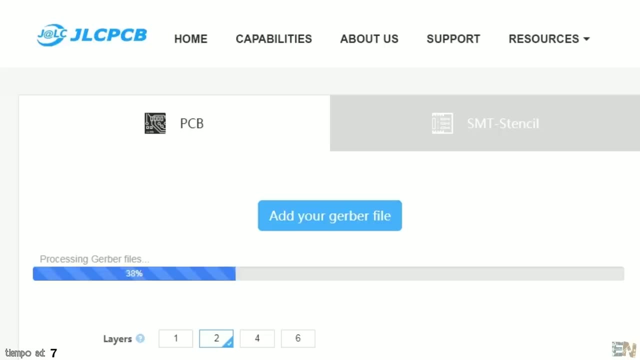 they are improving their services every day. Even this is your first time. ordering PCBs is very easy and all you have to do is to upload the Gerber files to JLCPCBcom. Select the settings that you want and you could get 5 PCBs of any color for only 2 dollars. 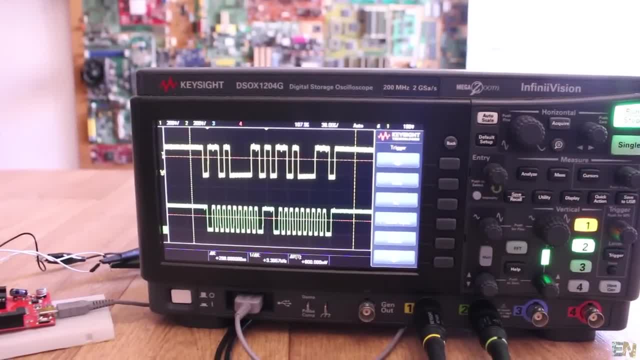 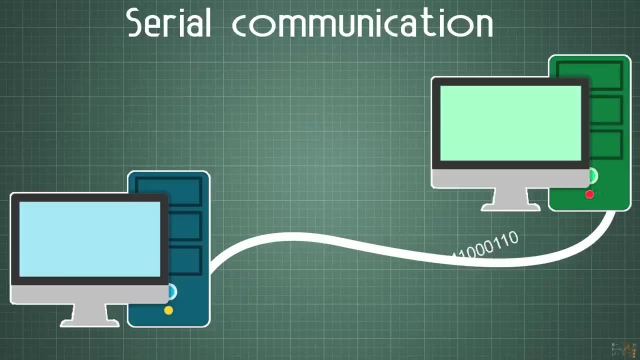 What's up? my friends welcome back. So what is a serial communication protocol? Well, it's a way of transmitting data in a line, one data after the other, and in this case we are talking about digital data. Imagine that you want to send the number 198,. 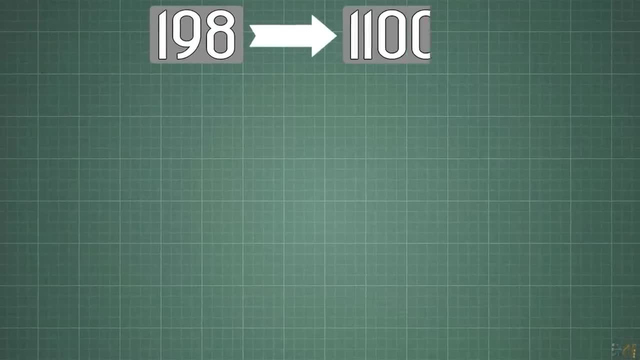 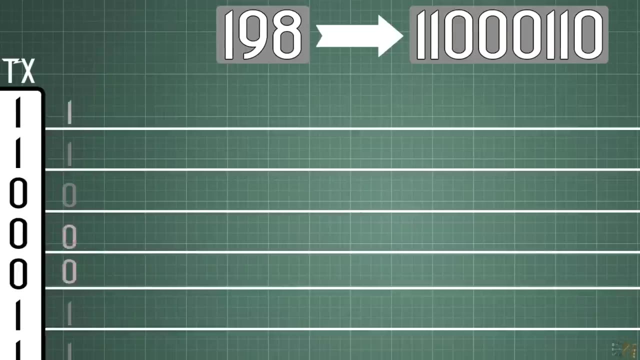 which in binary, which are just 1s and 0s, will be 11000110.. You could connect a wire for each bit and send the high digital pulse for 1s and the low value for 0s and do that at the. 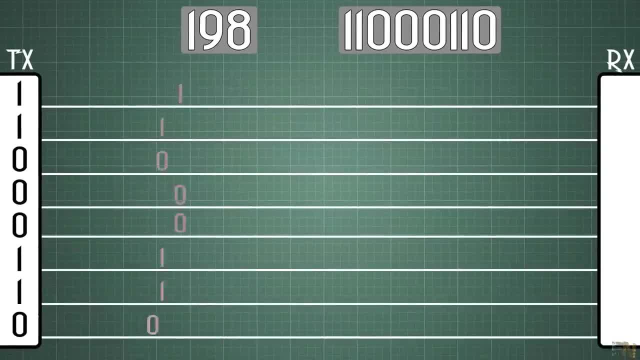 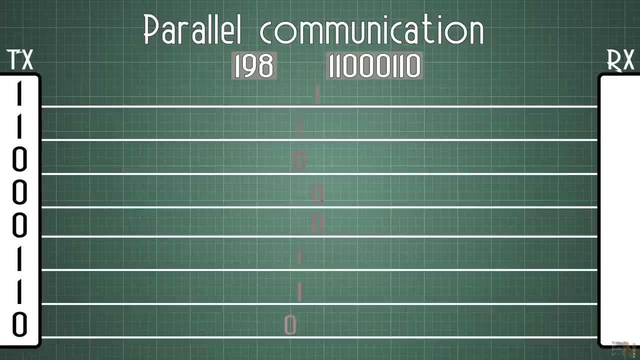 same time, So in just one moment you can send all the bits at the same time. This is called a parallel communication. The downside of this kind of communication is that we have to use 8 connections plus the ground reference, so a total of 9 cables. 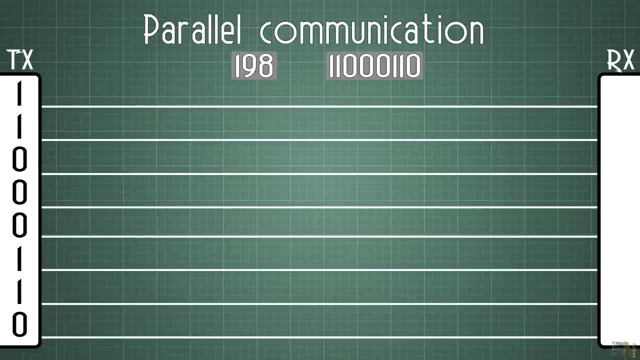 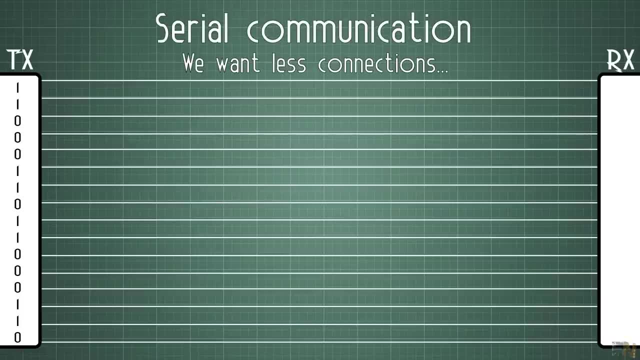 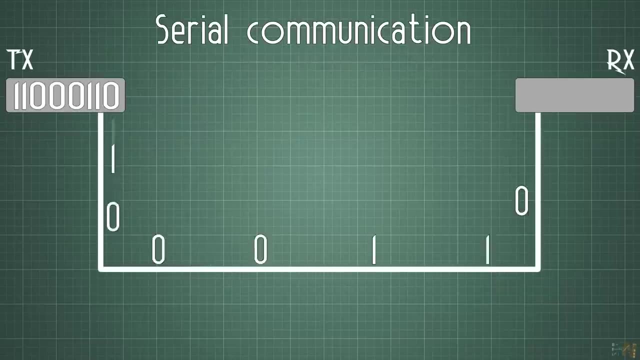 But this is for 8 bits. Imagine that you want to send a 16 bits data. In that case we will need 17 cables, and usually we want fewer connections. So instead of sending data each bit at the same time, what we will do is to place the bits in series and then we send each one. 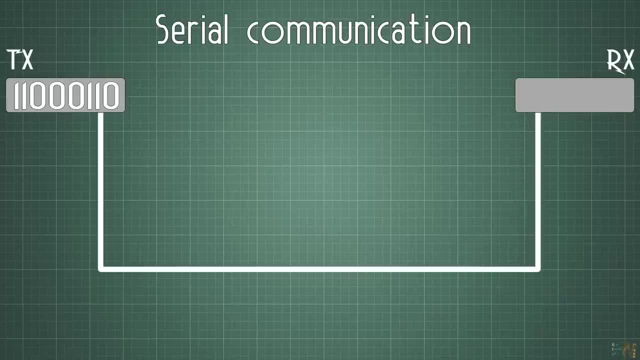 one after the other using just one cable. But you could already see the downside of this type of communication. If we send 16 bits in parallel, we need only 1 clock pulse to send all the data. If we send the same data using serial communication, we will need 16 clock pulses to. 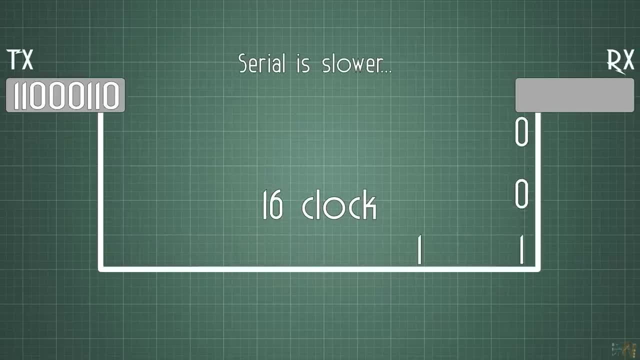 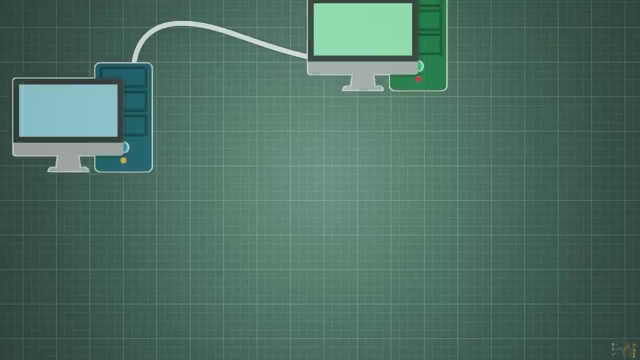 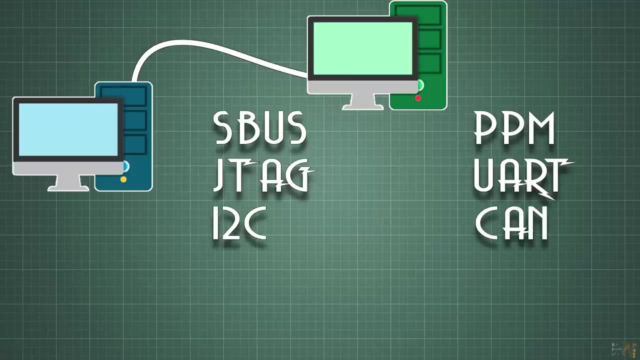 send the same amount of data, so this will be 16 times slower. So that's the main disadvantage. As examples for serial communication, we have the SBUS, the PPM, the JTAG connection, WART, I2C, the CAN, SPI, MIDI, USB, RS-233 and more, And even the Morse code could be. 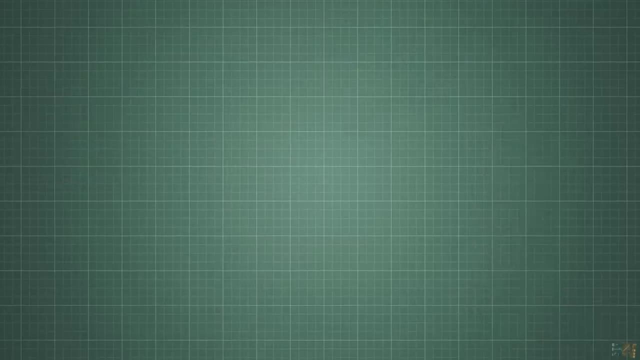 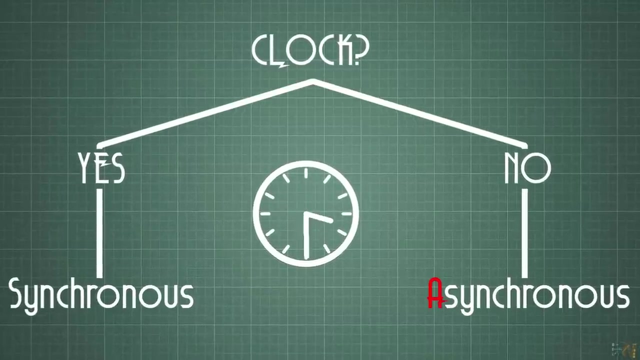 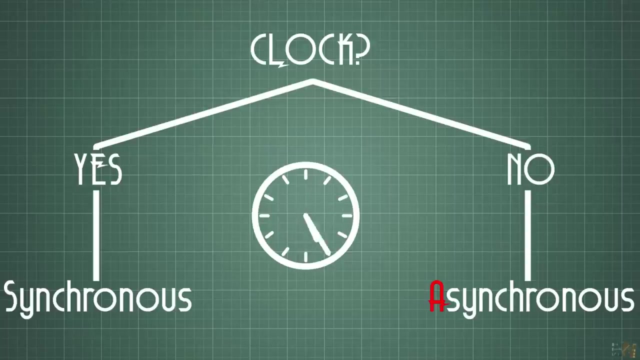 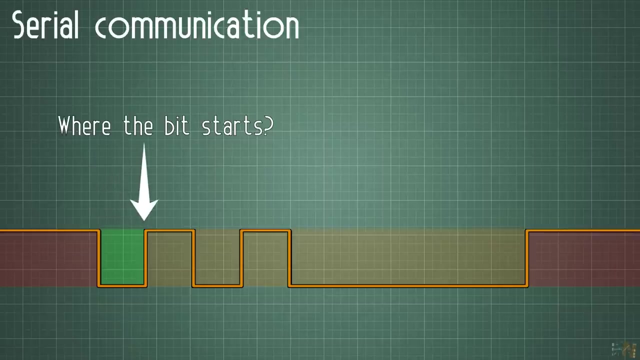 a serial communication. We have mentioned clock pulses before. Depending on this clock, serial communication could be synchronous or asynchronous, and the main difference is that one uses the clock to send the data at a specific speed and time. To understand that, we start with the most basic asynchronous serial communication. 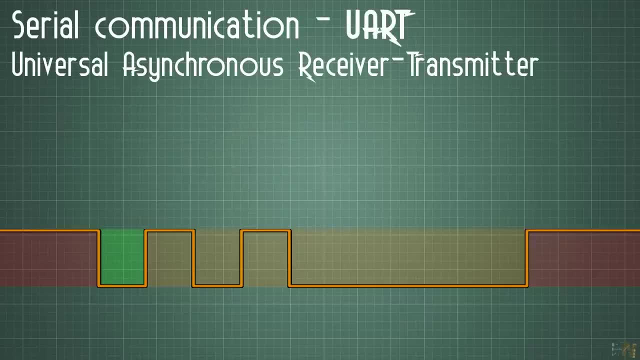 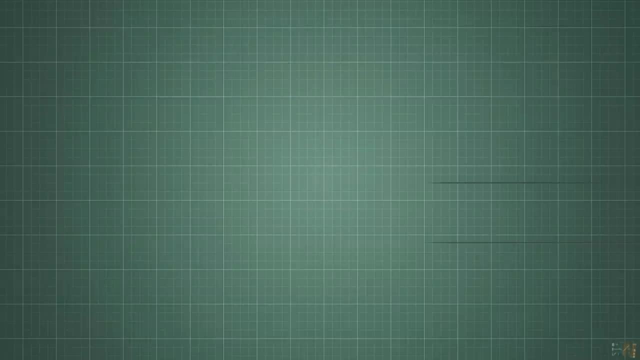 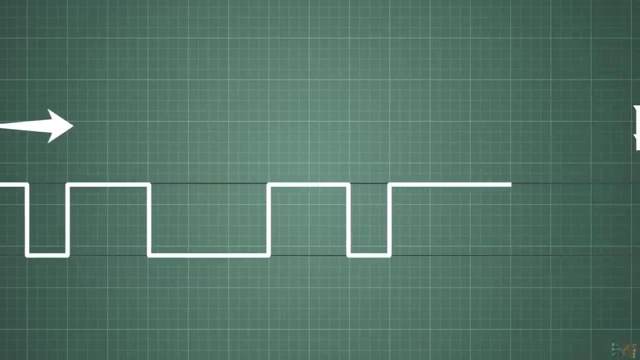 WART or Universal Asynchronous Receiver Transmitter. This type of communication uses only one cable to send the data plus the ground reference. The transmitter cable will be named TX and the receiver will be RX. The transmitter starts sending bits whenever it wants, So how does the receiver know when the incoming data starts? 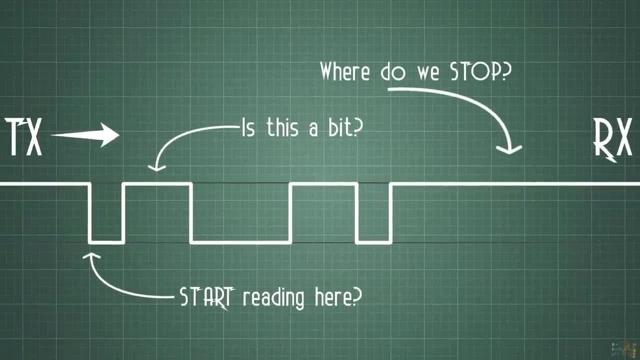 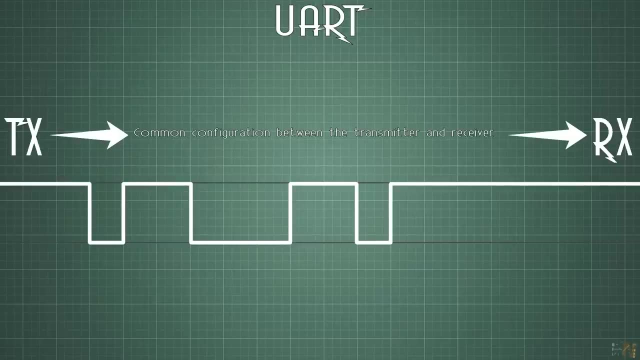 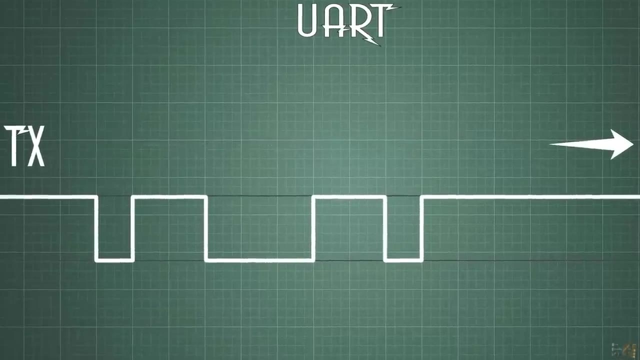 where it ends, when we have a bit or the other and so on. For that WART communication will need to place some common configuration between the transmitter and the receiver. Before making the connections you need to make sure that both the X and RX will work with the same settings. Three of these settings are the: 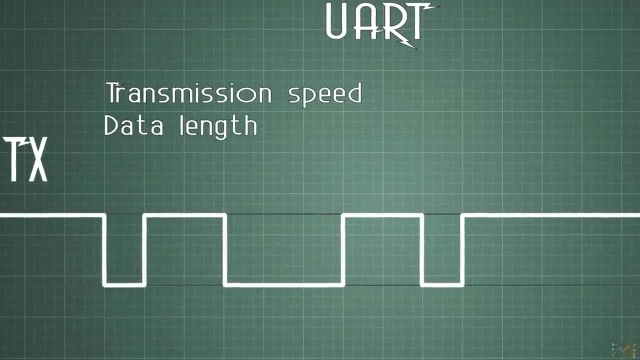 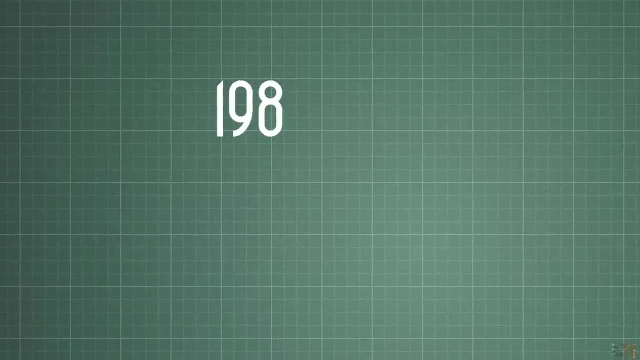 transmission speed in bouts per second, the data length in bits and how is the start and stop bit. So let's see what are these. Imagine that you want to send the number before 198.. The representation in digital pulses of this would be this one: 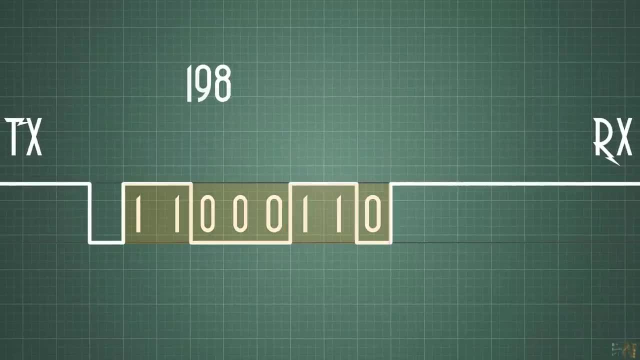 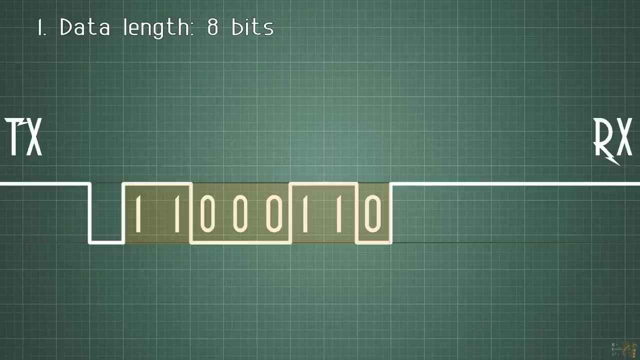 So with this data we already know that we will send 8 bits. So now we know the data length. The transmitter and receiver must have this same configuration. But if we analyze the WART signal, we won't see only these 8 bits. 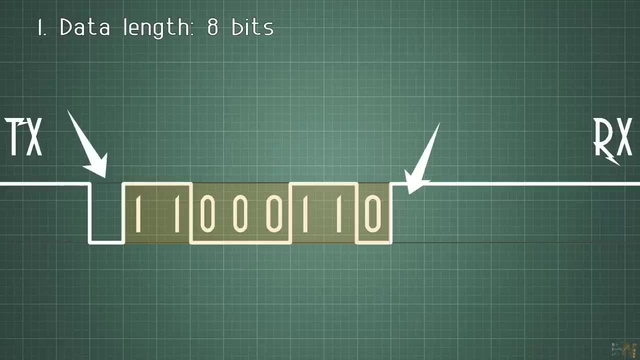 We will see something like this. That's because WART needs a start bit and an end bit. Usually the WART signal is always high and the start bit will be represented by a low pulse. So that makes it very easy for the receiver to detect when the data starts. 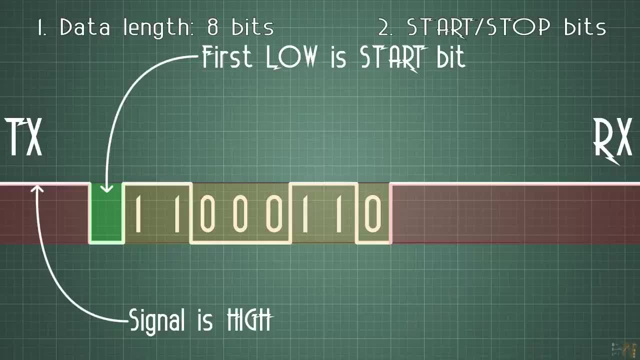 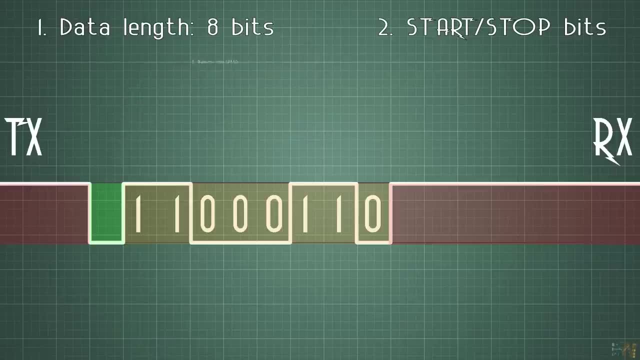 Each time we detect a low pulse, we know that we need to start reading the input data. Now here comes the 3rd configuration: the speed of transmission. Without knowing the speed, the receiver won't be able to know when one bit will end and the other one will start, and by that, 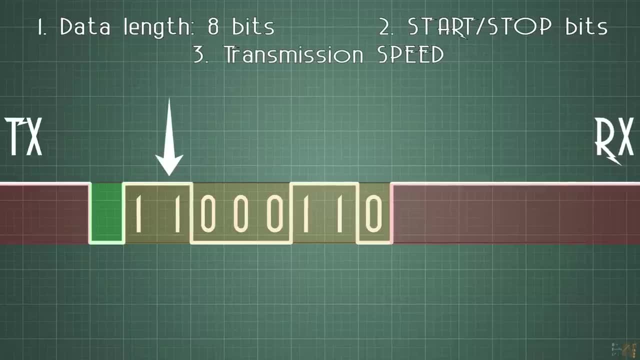 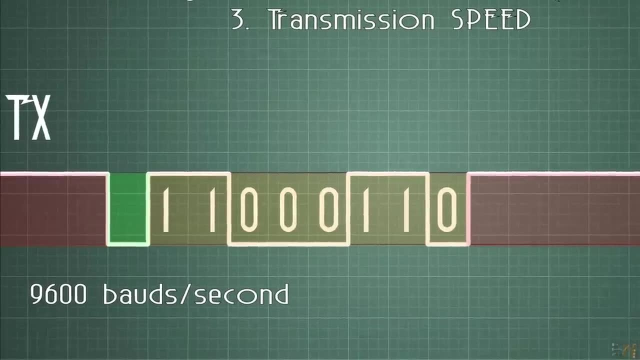 it will ring the wrong value. For that we need to start reading the input data. For that we need to. to set the speed in bps. A very common word, speed, is 9600 bps. that means the length of the bit will. 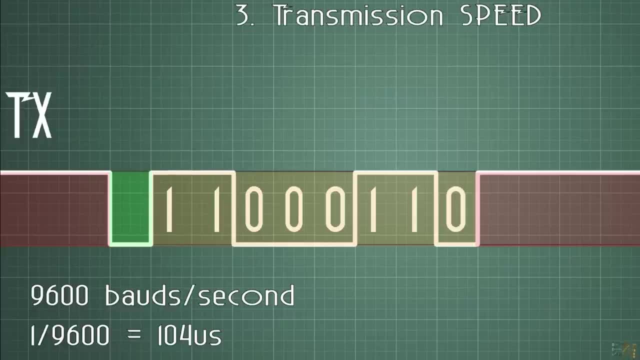 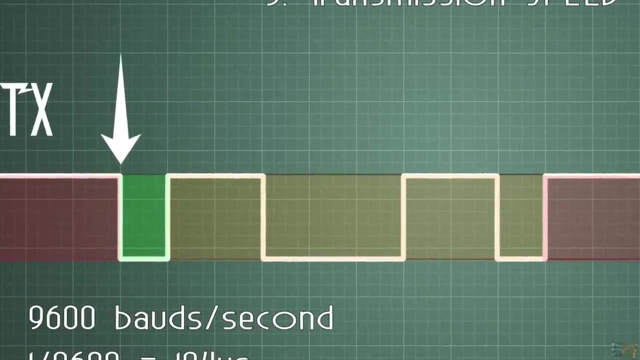 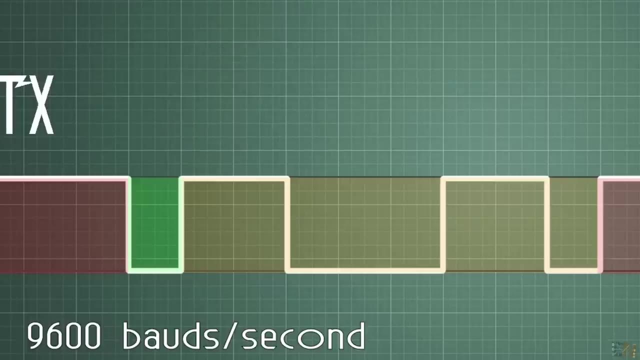 be 1 divided by 9600, and that equals 104 microseconds. So now all the receiver has to do after detecting the start bit is to count time. We count 104 microseconds and then we are at the beginning of the first input bit. But we don't usually save the value here because the data 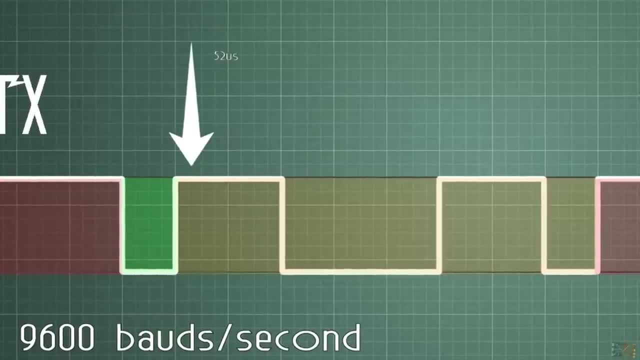 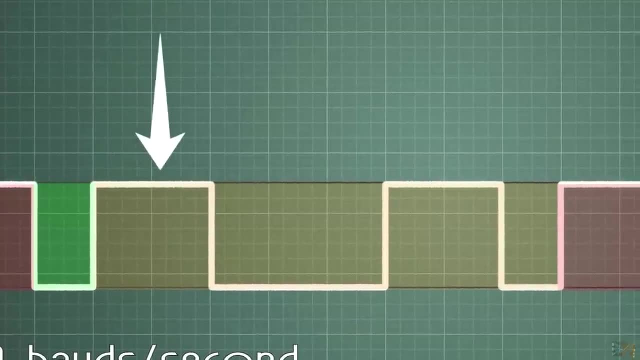 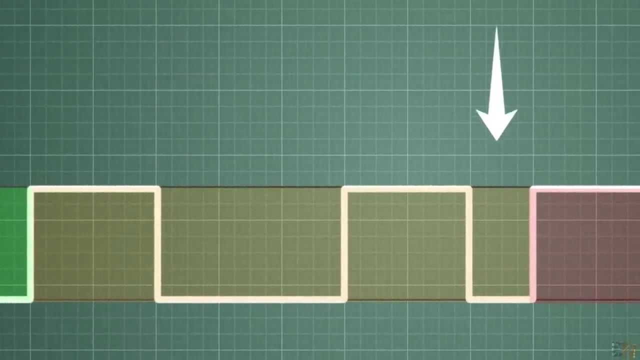 is unstable, so we will go in the middle of the bit. So we count 52 microseconds more Now, we save the first bit, and then we count 104 microseconds more and save the second bit, and so on. Once the receiver has all 8 bits, we'll wait for the stop bit, which is represented by a high. 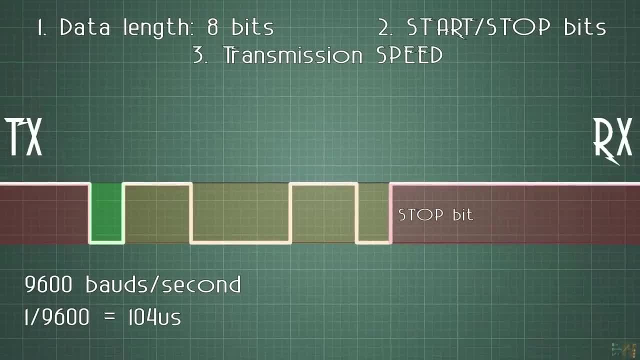 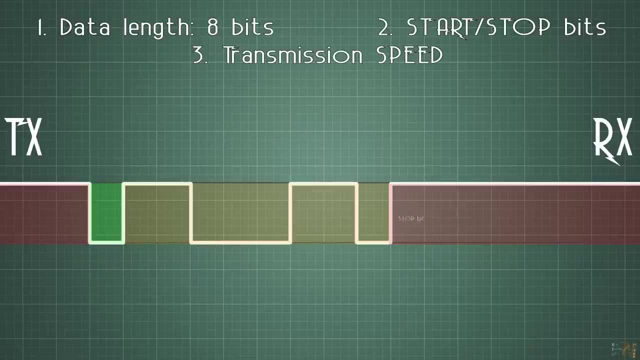 pulse, and then we can send the received data from the buffer to the rest of the system. This exact same setup could be made with different speeds or different amounts of bits for the same data. Usually the start and stop bits are always like this: So that's how the WART communication works. 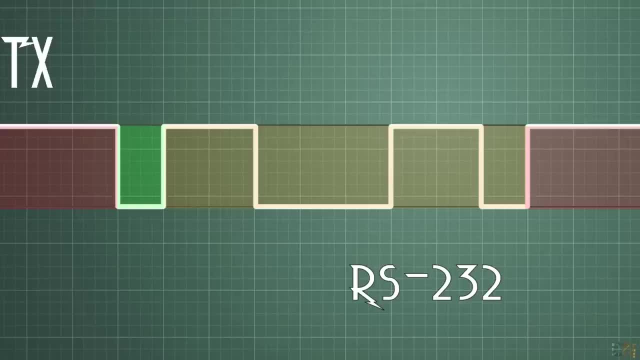 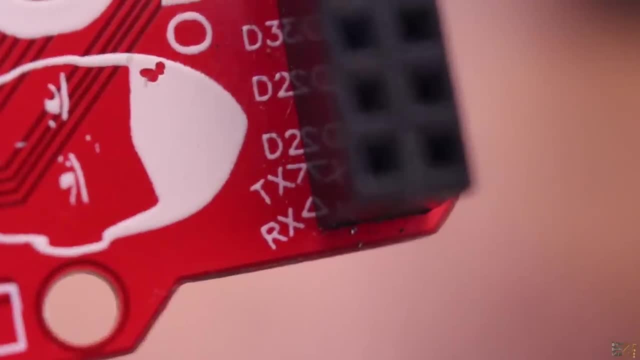 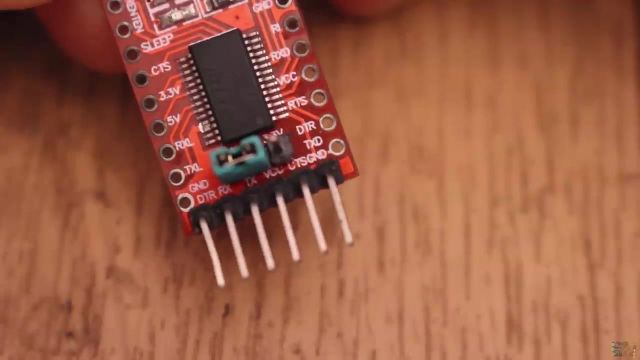 Another version of the WART communication is the RS-232 that is used by old computers. The Arduino, for example, uses the WART communication to upload the codes or send the data to the serial monitor. This right here is a WART chip, and you will also see that it has a DTR pin and sometimes you will see a CTS pin. 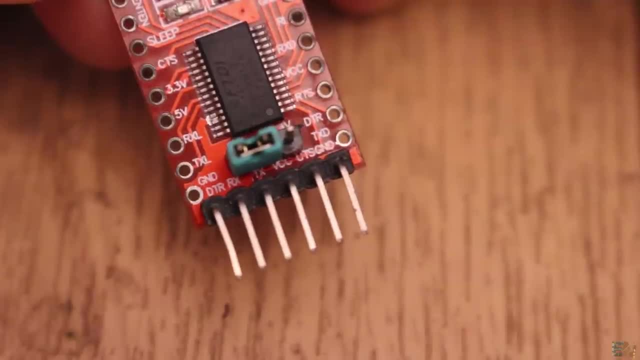 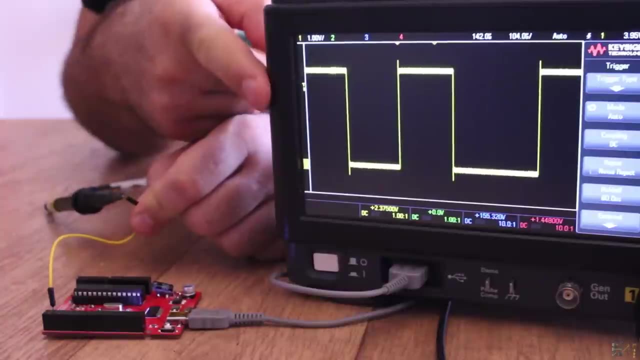 These pins are used to notify that the data terminal is ready and that the receiver is clear to receive, so in this way we won't have flow problems. I connect the Arduino and here I have the WART signal on the oscilloscope and right now I'm sending the number before 198.. As you can see, we have exactly the. 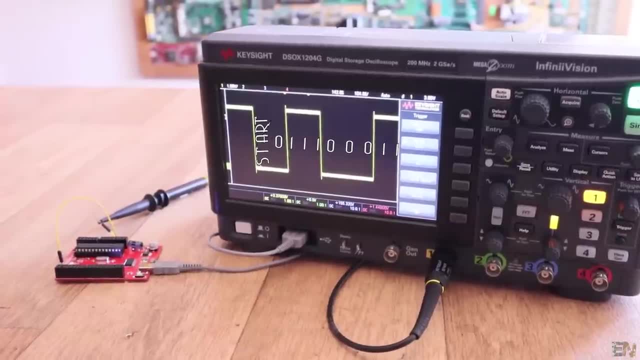 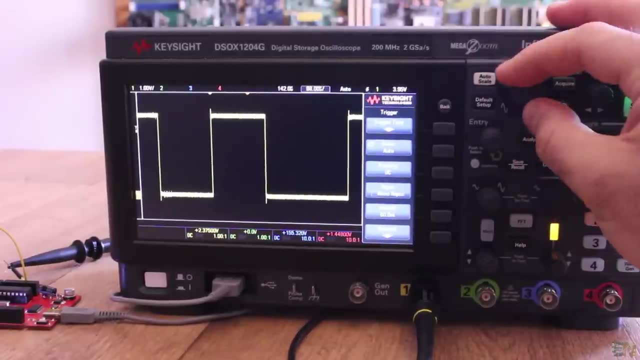 representation before The start bit, the data and the stop bit and the rest of the time the signal is high. Usually, devices will have both the TX and RX pins, so they could both send and receive data with the same protocol. Okay, guys. next we need to take a look at the first synchronous and 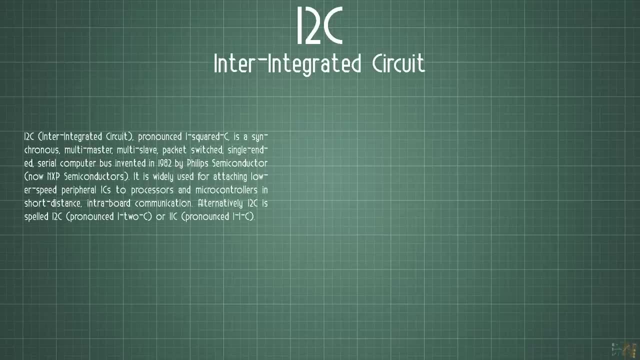 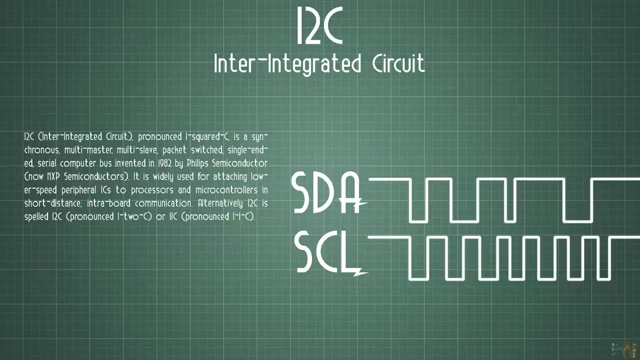 serial communication, and this is the I2C or the inter-integrated circuit. This protocol was developed by Philips and in this case we need two connections plus the ground reference. One wire will send the data and this will have the name of SDA. 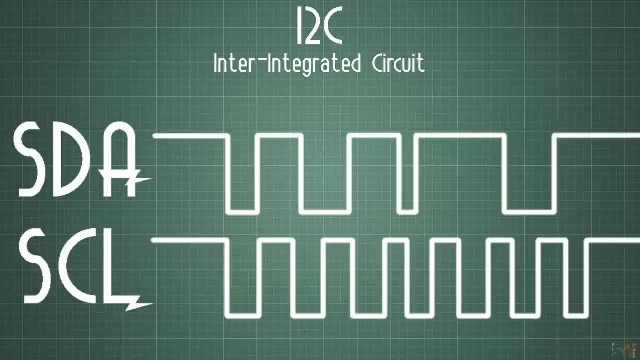 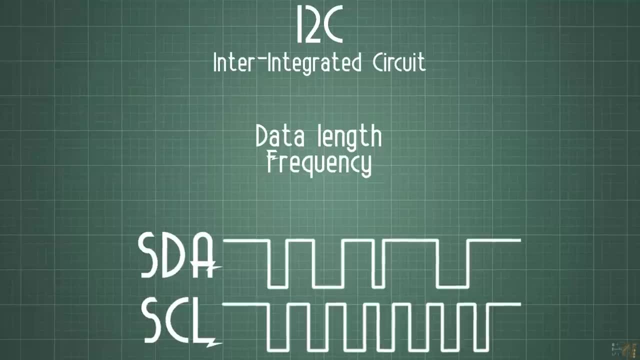 and the second wire is the clock, because this is asynchronous communication and it will have the name of SCL. Once again, we need to specify the amount of bits that we will send and also to know the clock frequency for both the transmitter and receiver, Usually I2C. 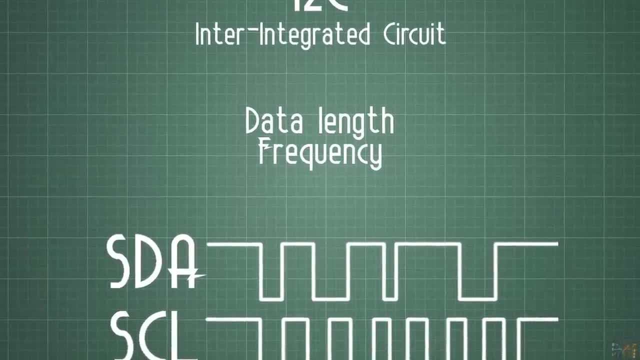 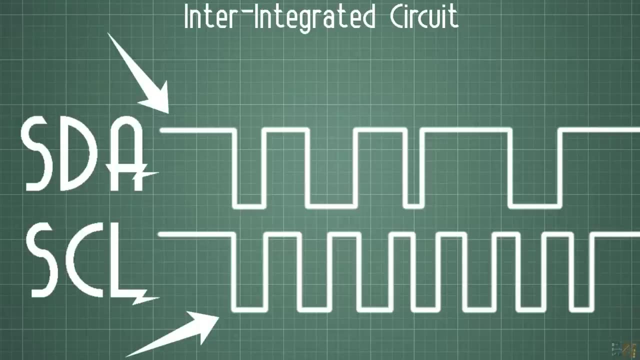 works with speeds up to 400 kbps and it will send data of 15 or 16 bits In this case. at the same time we send the data, we also create a clock pulse with the same frequency as the bits of the data, so the receiver will know exactly when one bit 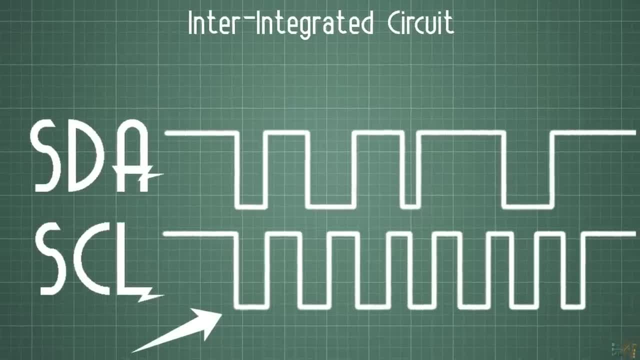 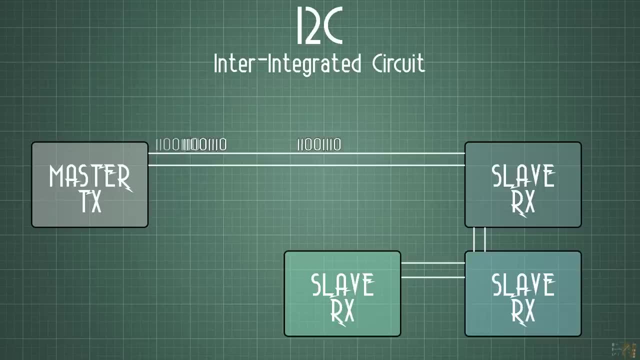 will end and the next one will start, so this can go faster, since we don't need to count the time. as in the WART communication, Also using I2C, the transmitter will send all kinds of data, but only certain receiver will be able to save the values. 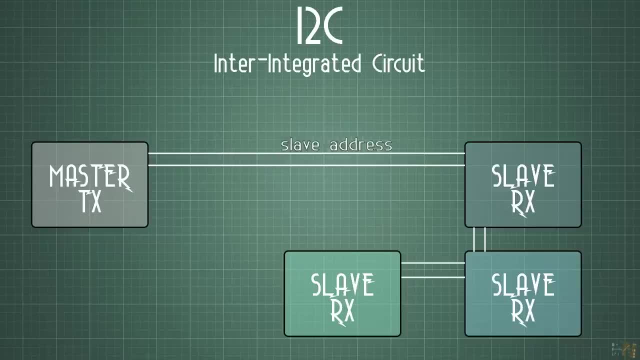 We do that when we send data to the transmitter, We don't have to do the same thing for the receiver, so we can send data as many times as possible, but the receiver will be able to save the values. We do this that with the use of the slave address. Each receiver will have a different slave address. 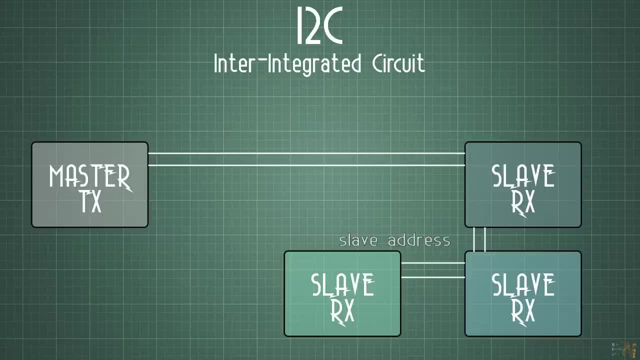 So the transmitter will first send the address, which for example could be 68, then it will send the data. Only the receiver with the 68 slave address will store the data into its buffer. The WAD communication is a one-to-one communication, but the I2C could. 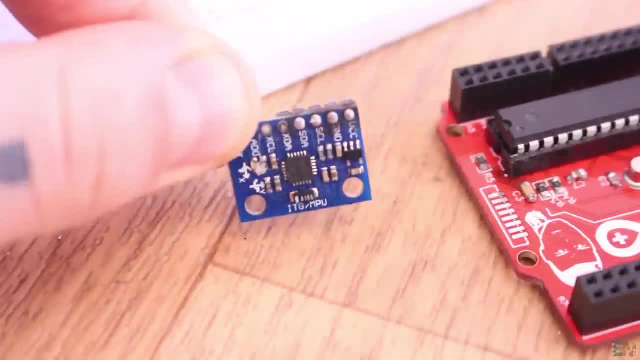 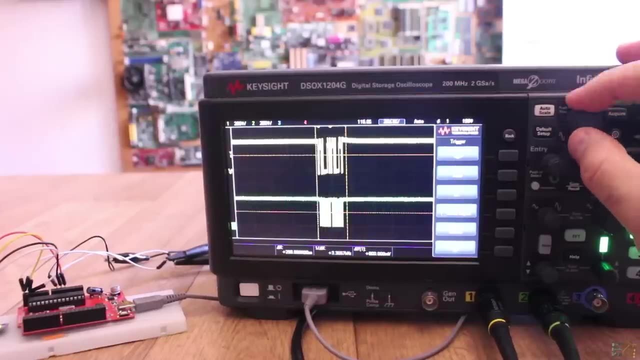 be used with multiple receivers. For example, this MPU6050 module uses I2C communication. I connect my oscilloscope to the data and clock pins and now we can see the signal on the oscilloscope. As you can see, we have a squared signal as a clock and then we have the send data. 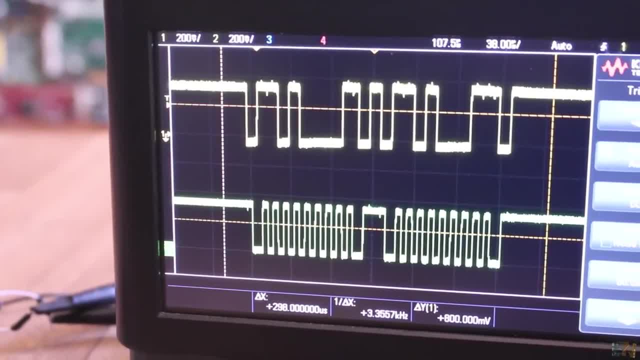 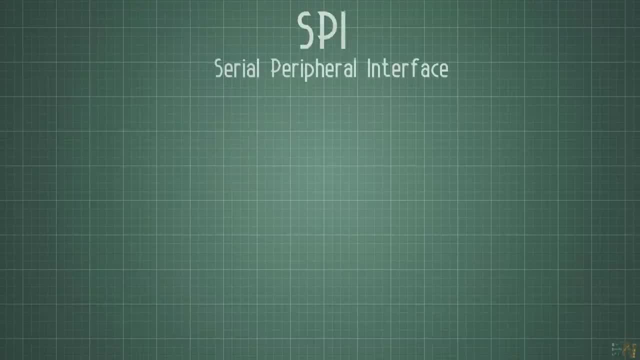 Each time we send a new value, we also enable the clock signal and also send the slave address before sending the new data. That was I2C. Finally, let's take a look at another synchronous serial communication, SPI, or Serial Peripheral Interface. 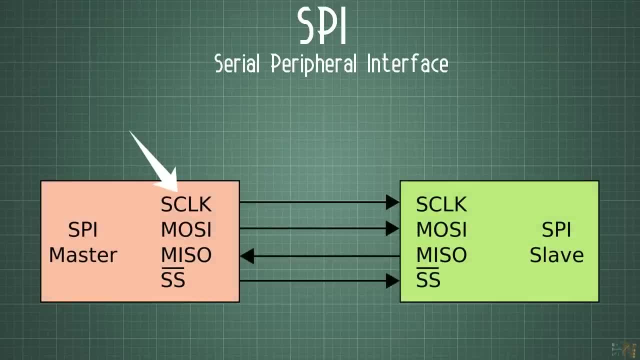 In this case we still have the clock connection, but we also need 3 more wires: MOSI, which is the master output, slave input. MISO, which is the master input slave output, and the chip select wire plus the ground reference, So using a total of 5 connections. 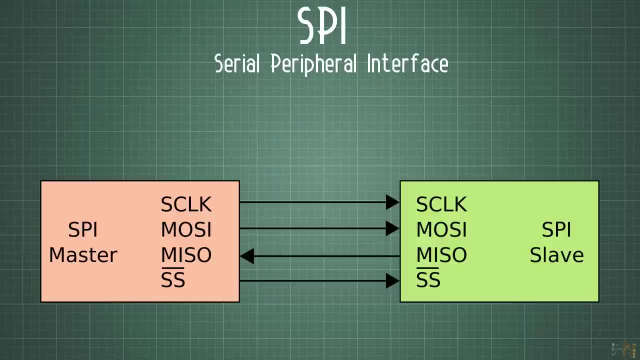 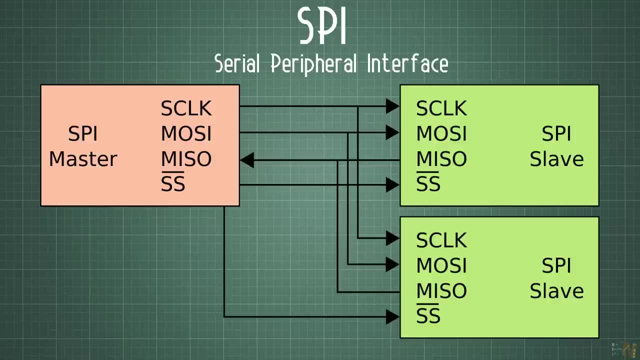 we could send the data Once again. we have a master transmitter and a slave that could receive the data. The MOSI wire will send the data to the slaves, but the master device could also receive data from the slaves using the MISO wires. In this case, we don't use a slave address. 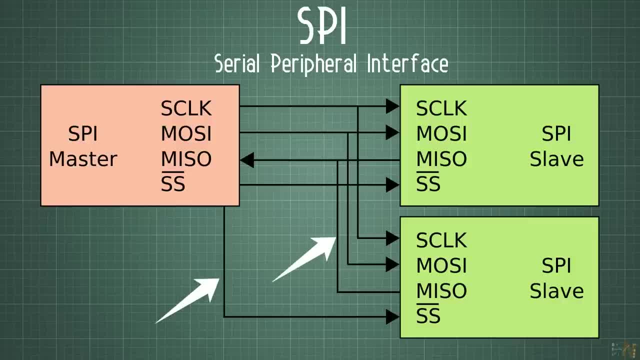 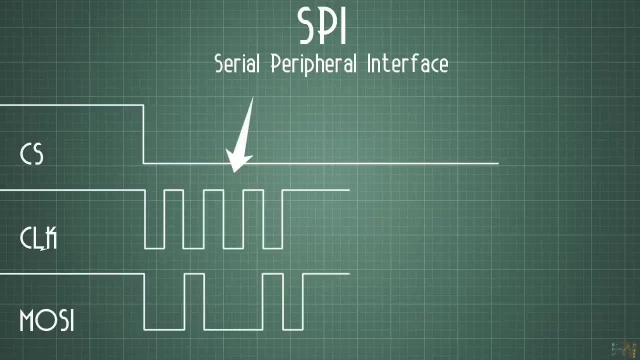 as for the I2C, Instead of that we have the chip select To start a new transmission. the master will put the chip select pin to low and then we send the clock and data signals. So if you want more slave devices connected. 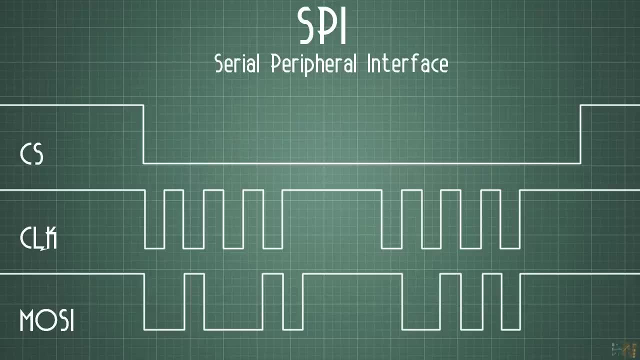 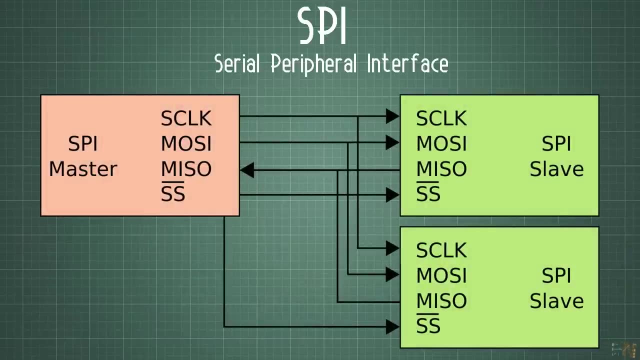 you will need a chip select connection for each one. The advantages of this type of communication is that it's full duplex. In a full duplex mode, both devices can transmit the signal at the same time, so we could both send and receive. We can't do that with I2C, because that is a simplex. 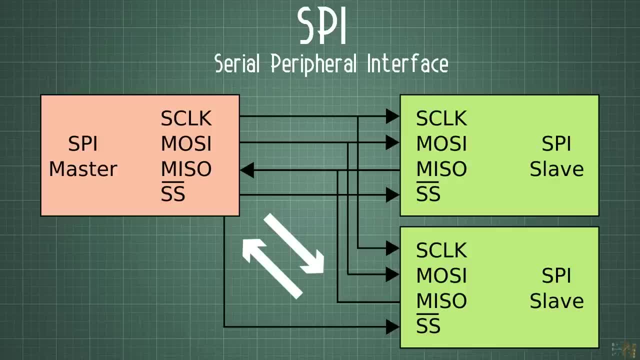 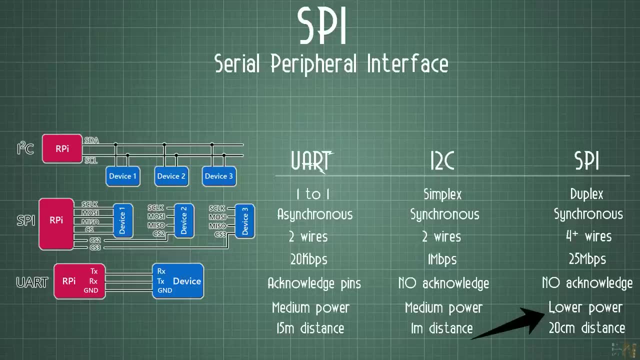 communication Also. at the same time, the speed of transmission for the SPI is way higher than the I2C or WART communication and at the same time the power consumption is also lower. We can set the amount of bits that we want to send in the 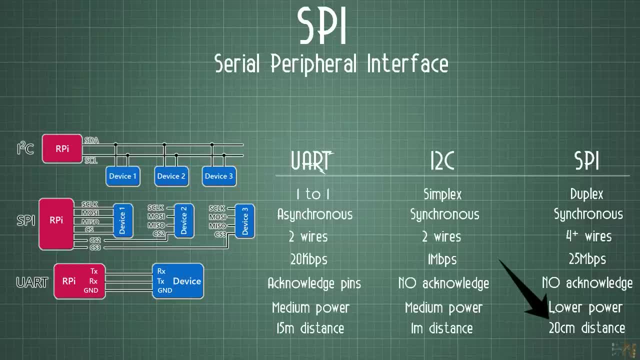 code, but unfortunately this communication can send the data for long ranges, as we can do with the RS-232 or the CAN bus. Also, these communications have no acknowledged pins, so the master could send the data even if you don't have a slave connected, and the data won't. 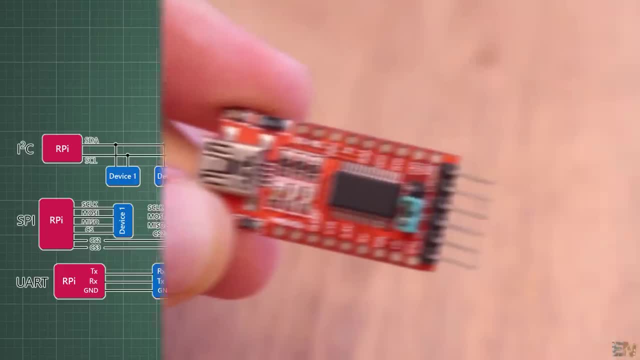 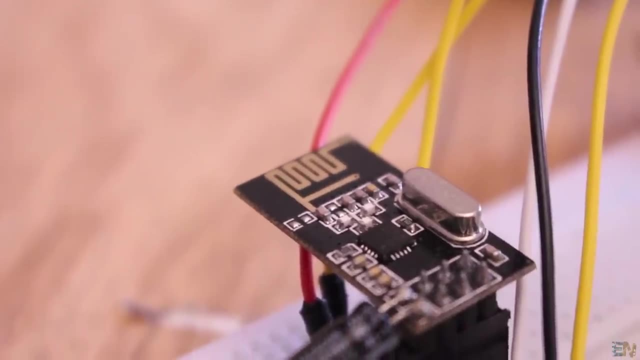 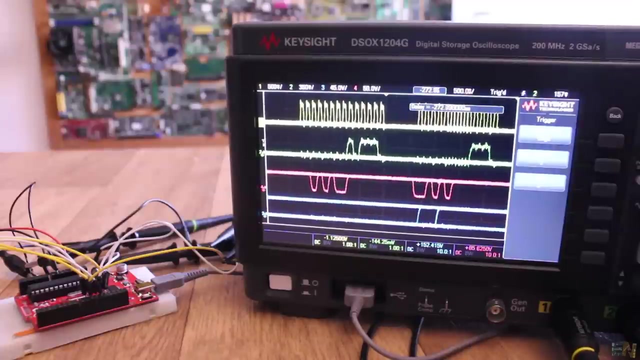 be received by any device. In case of the WART communication we could have the DTR or CTR pins. Now this NRF24 radio module uses SPI communication. I connect it to the Arduino and hook up the oscilloscope. We can see 4 signals for clock, MOSI, MISO and chip select. As you can see.